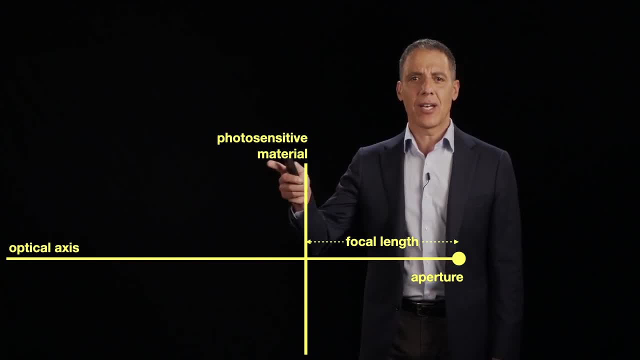 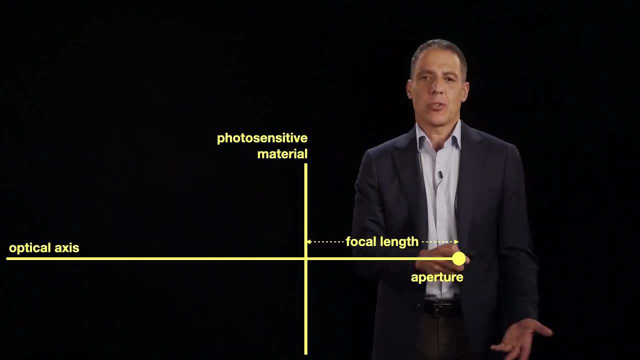 So, first of all, I've got the photosensitive material here, I've got the optical axis going out this way, so the world is here. But notice now that the aperture is behind the camera, which of course makes no sense and in fact is not physically plausible. 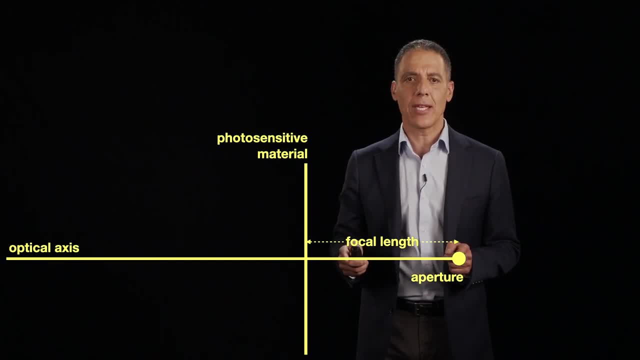 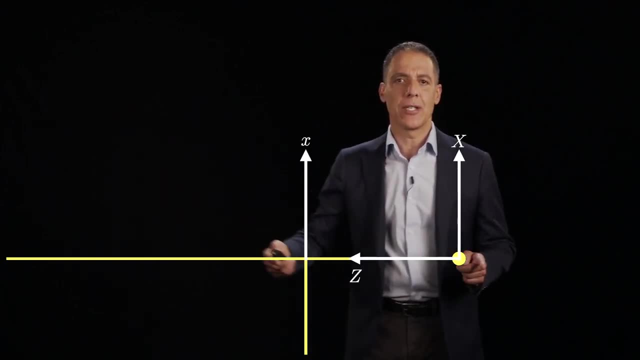 But you're going to see in a minute why I've done that. So I've got still the same focal length, the distance between the aperture and the photosensitive material. I've got my optical axis going out, so I'm going to put a point out in the world here. 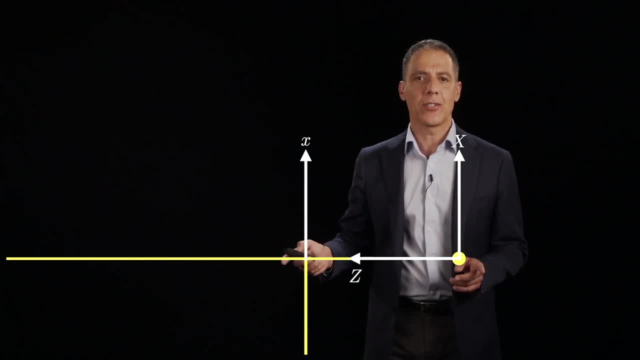 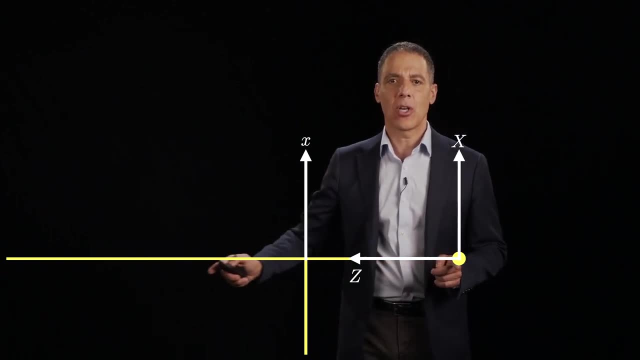 And let's see what happens. Well, let's first define our coordinate systems. So I've got my world coordinate system, which looks exactly the same as before. I've got the z-axis going out along the optical axis, starting, by the way, at the aperture. 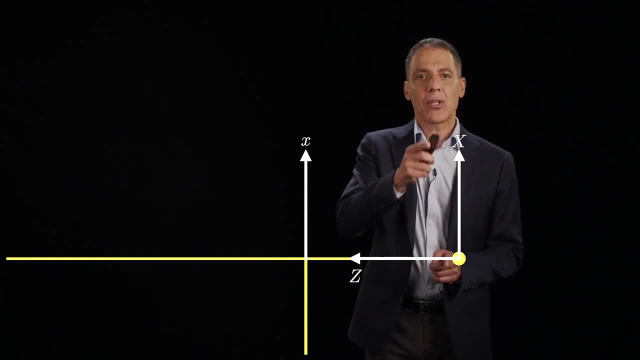 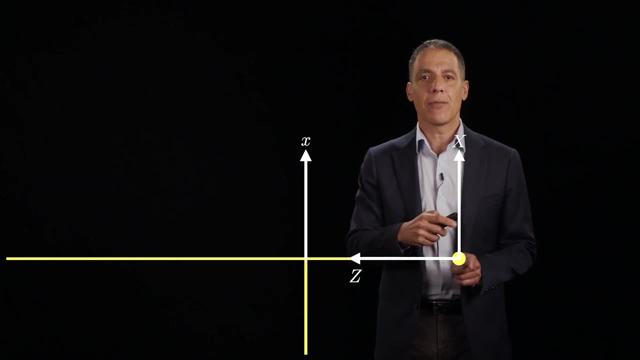 That's where we're always going to be starting. I've got the capital X still in the world coordinate system going up and parallel to the photosensitive material, And then, of course, I have my photosensitive material, which has a small x-coordinate system. 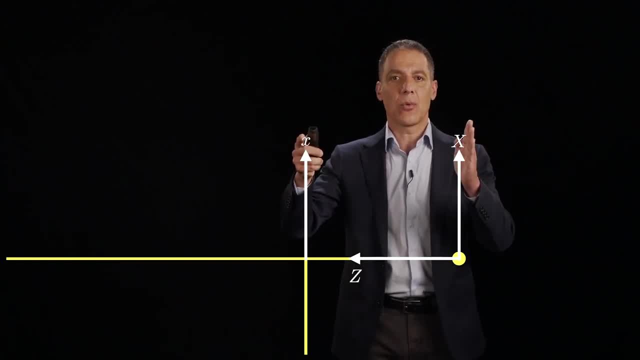 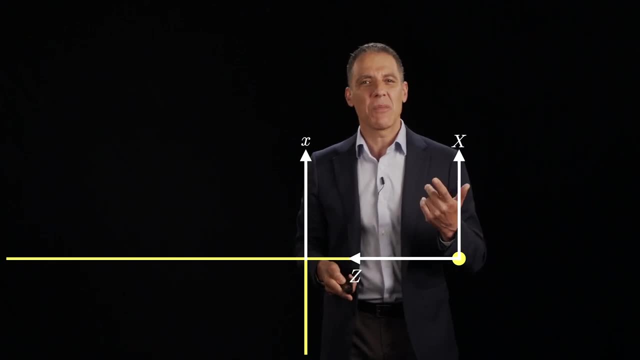 Again. origin: I've got the optical axis and it's parallel to the world over here, So the pieces are exactly the same. What have I done? I've just flipped these two. Why have I flipped them? I'm going to get rid of that negative sign in the perspective projection. 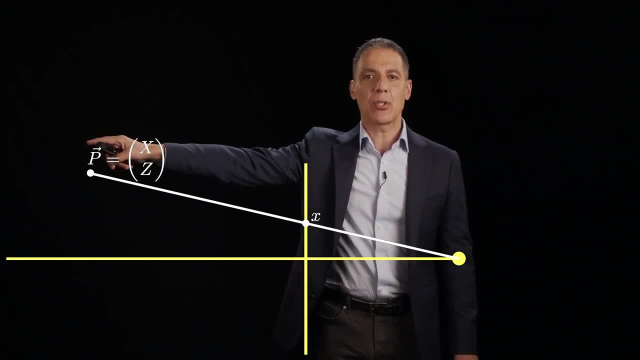 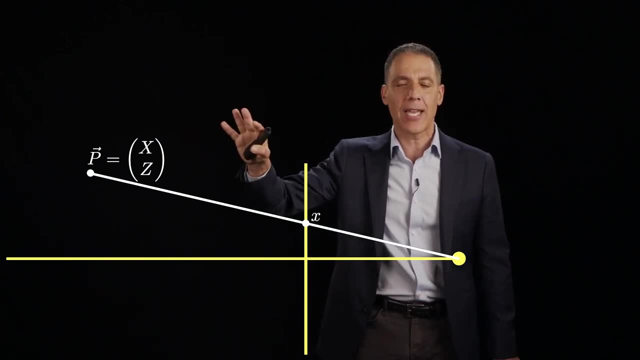 Okay. So let's take a point out in the world, capital P, vector again, capital X, capital Z, We have a point, a two-dimensional point. We're still in flat land, We're still in two-dimensional world. We'll do 3D later. 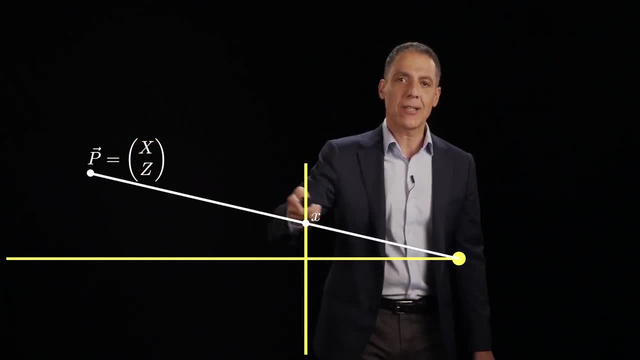 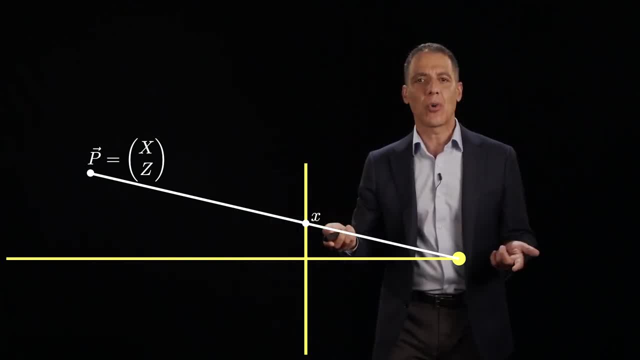 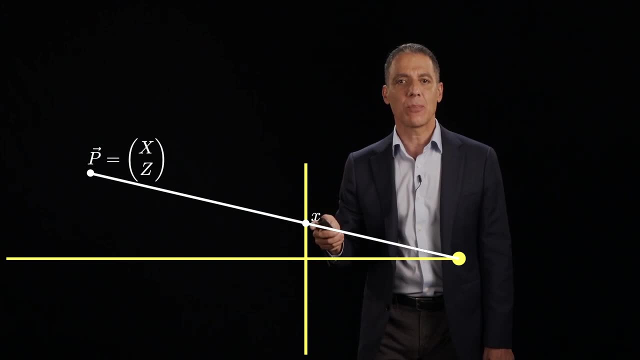 Again, not physically plausible, but this is the way people draw these cameras, because it slightly changes the perspective projection model. So there's my little x. That's the projection of the point onto the sensor. Now, if there is any sanity in the world, this should end up looking exactly like the perspective projection that we've already seen, minus the minus sign. 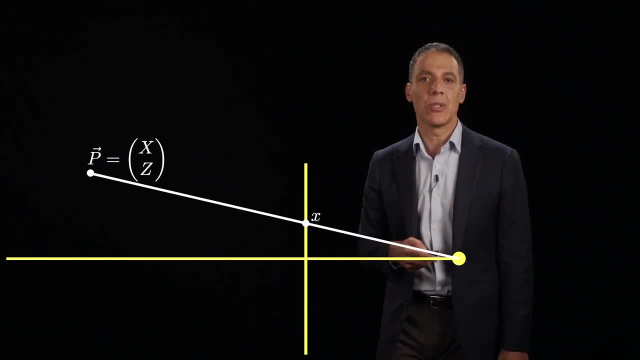 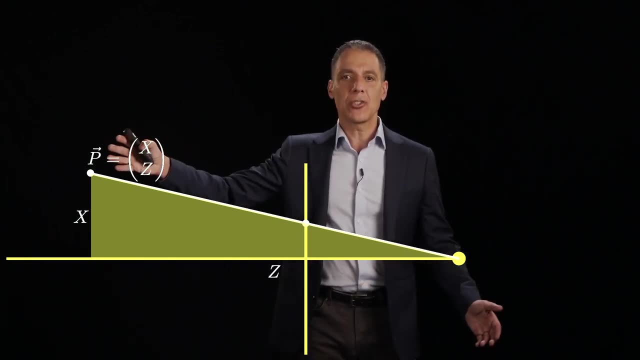 Well, Well, let's go ahead and derive that instead of me just promising you that is in fact, the case. All right, Triangles are our friend geometry. So what do I have here? I've got one big triangle that is made up of the aperture, the point in the world, and then the corresponding point on the optical axis. 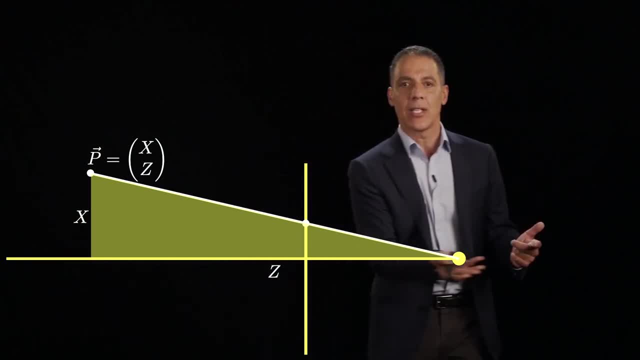 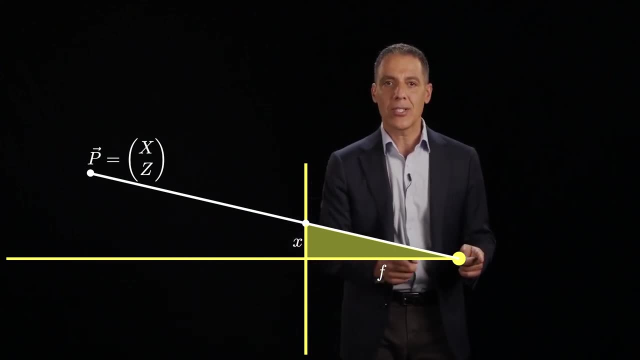 So the triangle has sides capital X and capital Z. I have another triangle, a smaller one, right here, little x, And then what is this distance here? Well, that's just the focal length. And so now I have two similar triangles. 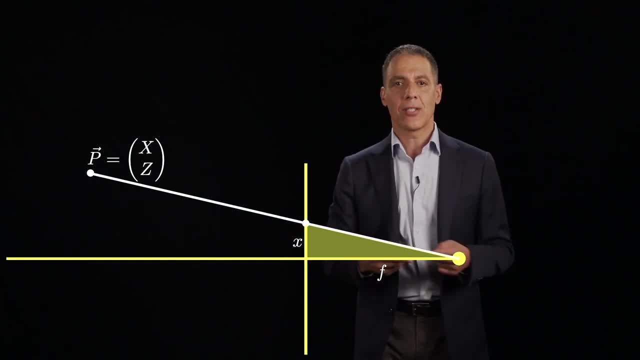 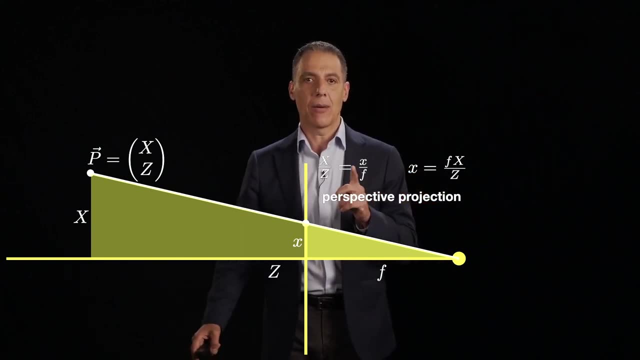 And now I can play the same game. The ratio of the height to the length should be the same. So now let's go ahead and look at that. So what do I have here? I have that. Let's go over here first. 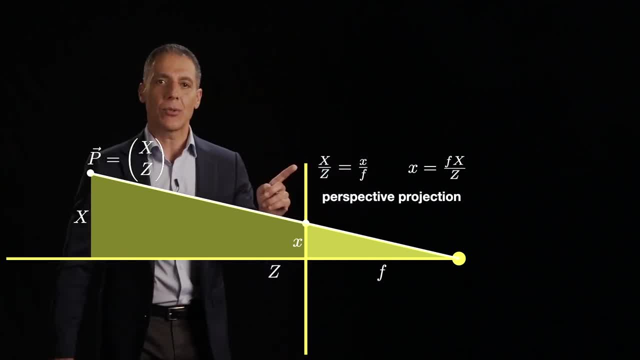 I've got capital X over capital Z is equal to little x over little f. Notice there's no minus sign. Why is there no minus sign? Well, notice here that I have a positive big X and I have a positive little x. And if I invert it? 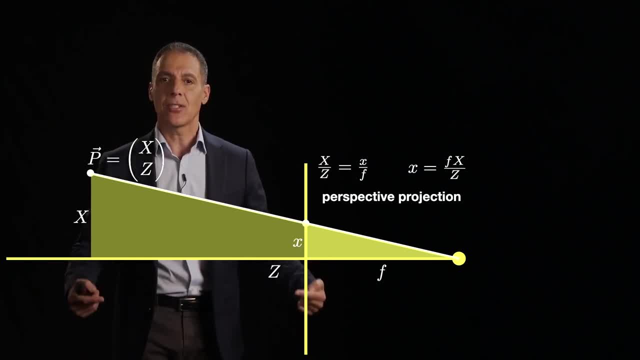 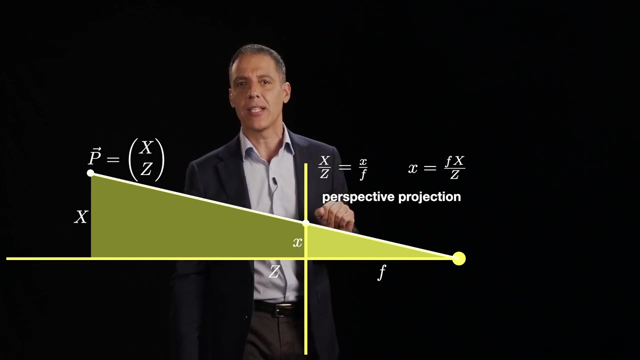 I would have negative big X and negative little x, And so there's no inversion here, because I flipped the sensor and the aperture, And so now what I can write is that little x is equal to fx over z, Same perspective projection equation. We've just dropped the negative sign. 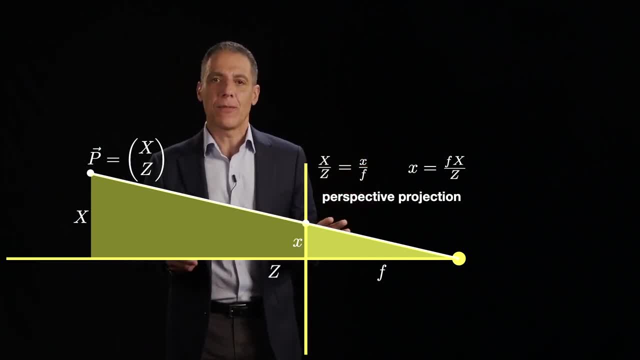 And again, the reason I do this is not that it's really fundamentally any different. It's that in the literature you will often see perspective projection written without the negative sign, and all they're doing is essentially doing the inversion that you're going to do anyway. 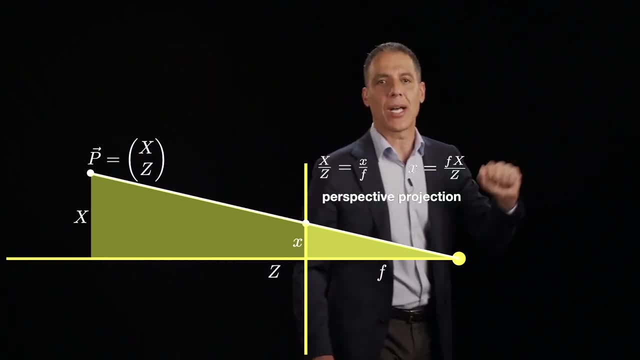 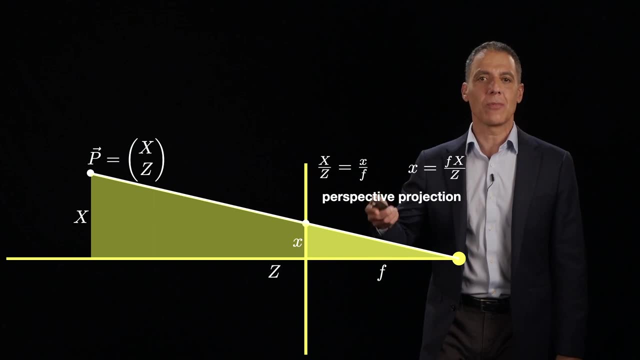 They're just doing it directly in the model instead of having to do it in a post-processing step. OK, so everything's still the same. Everything is inversely, the size of everything is still inversely relationship related to z And we have the same basic effects. 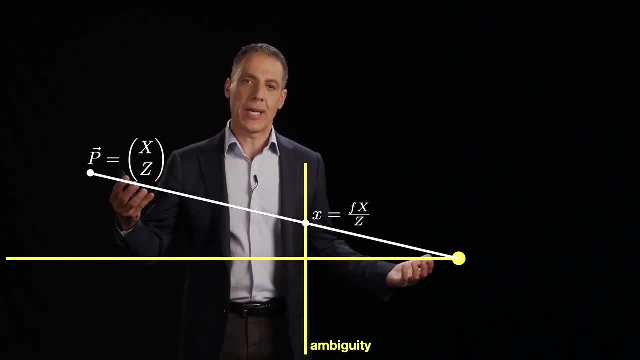 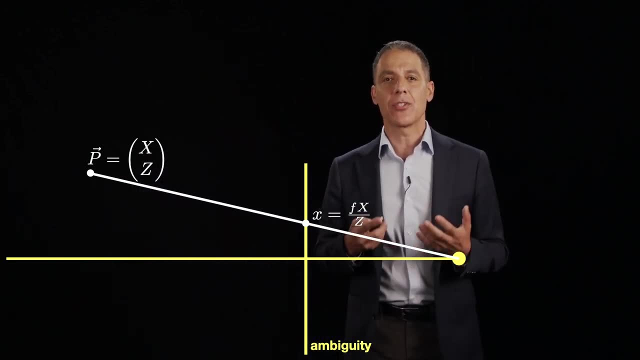 Now, something really interesting happens when you, when we have this perspective projection model, whether it's this one or the inverted one, And it gets at in some ways why computer vision is so incredibly important, And it gets at in some ways why computer vision is so incredibly hard. 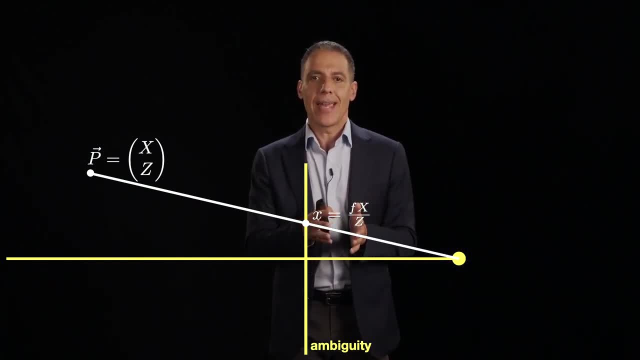 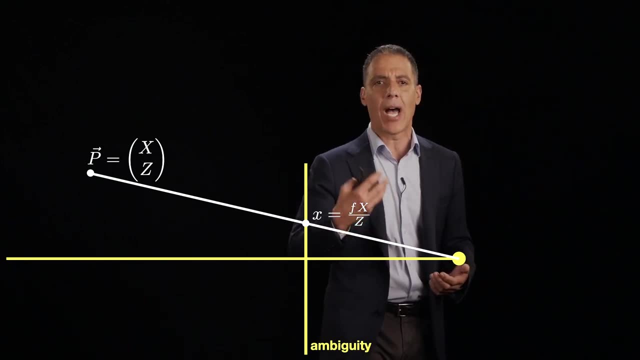 You have this sense when you look at an image, that it's a pretty good representation of the world. It's not. I'm not confused by what I'm looking at. I can reason about things. I know that there are objects there. I know their relative sizes. 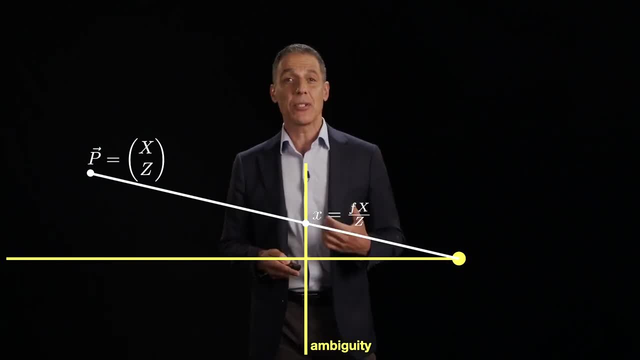 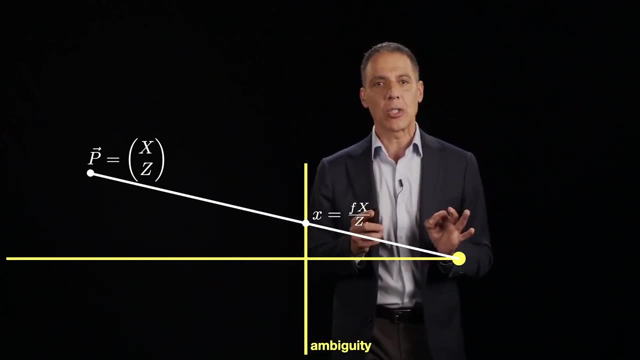 I know about where they are to each other. I can recognize things, But there is a phenomenal amount of ambiguity in these images. that may not be immediately apparent, And I want to point that out because it is arguably one of the things that makes computer vision very, very difficult. 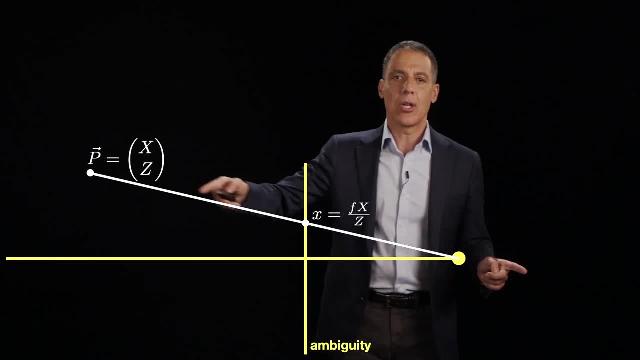 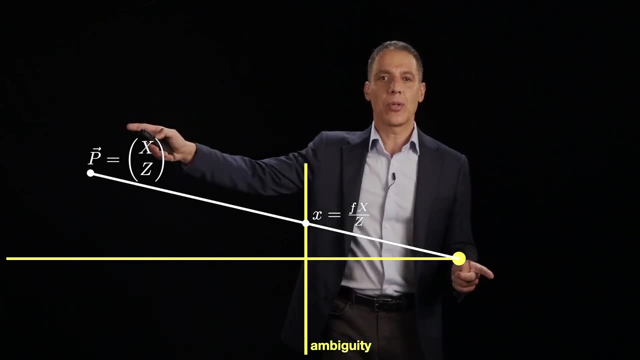 So let's again Start with a single point out in the world XZ, We now know that the projection into the sensor is going to be little f focal length times the X coordinate of the point in the world divided by the Z component, which is of course again the perspective projection. 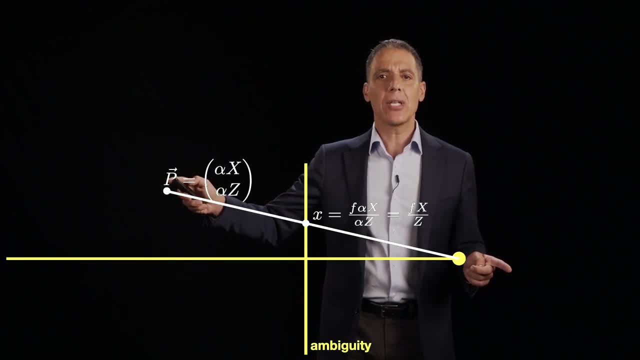 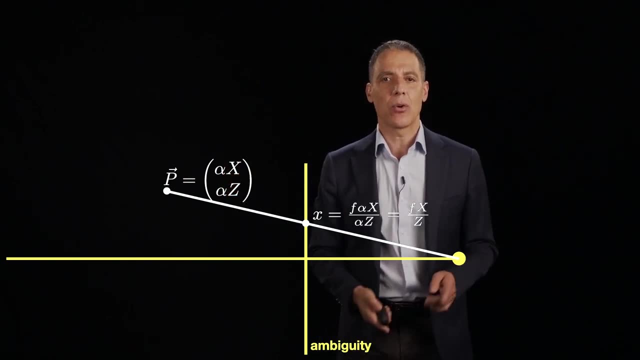 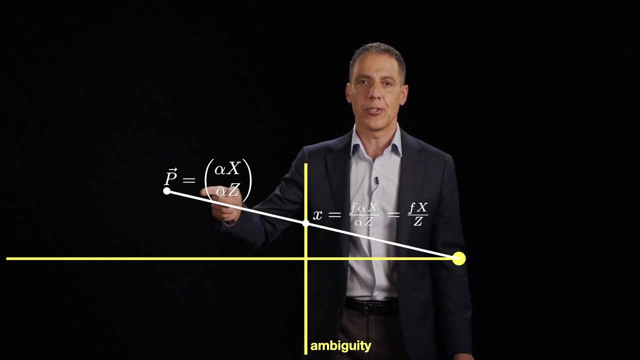 Let's think about another point that is along this ray. So let me call that point alpha X over alpha Z, And so notice that I've scaled the X and the Z component by exactly the same scalar value, alpha, And that of course just moves the point along the line through the origin. 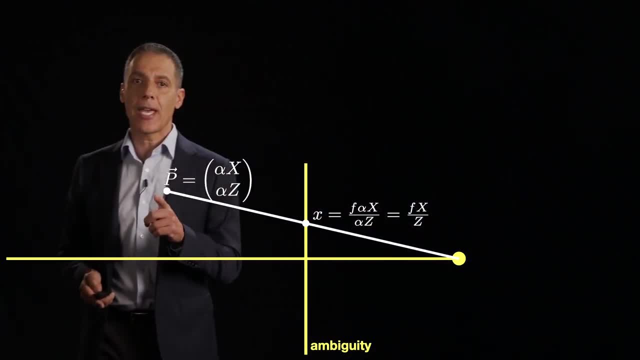 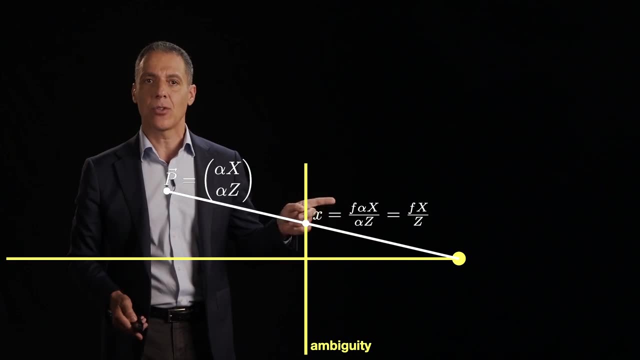 And notice now that that point, which is much closer to the camera, projects to what? Well, it's just f, alpha X over alpha Z. The alphas, of course, cancel And I'm left with fx over z. It's exactly in the same position as the point that was further out. 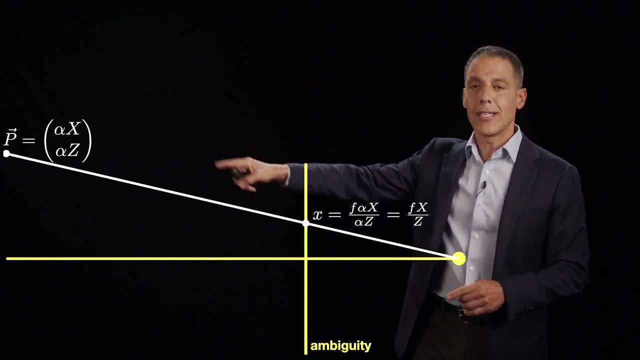 And, of course, if I take a point and I move it even further out, it's at some other alpha X, alpha Z, And it's going to move, And it's going to move, And it's going to move, and it's going to project to exactly the same point. 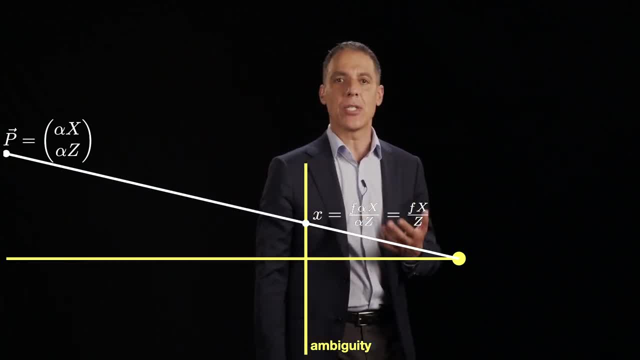 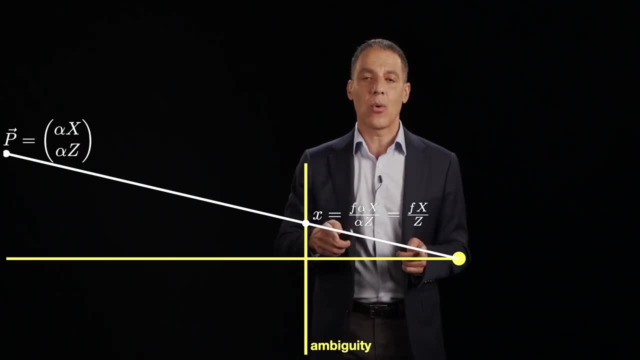 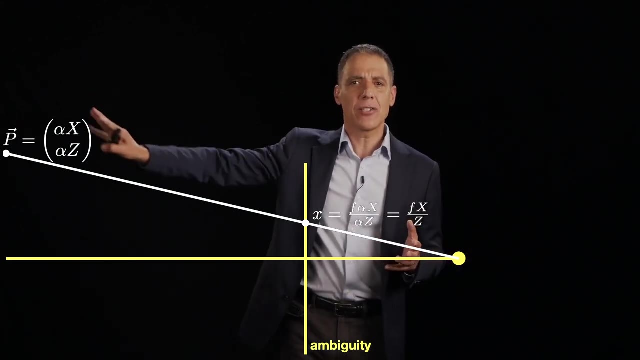 which means that we have an inherent ambiguity in the image formation process. All points along this ray will image to exactly the same point, And you sort of knew it had to be that way. Why? Well, because I have points out in a two-dimensional world. 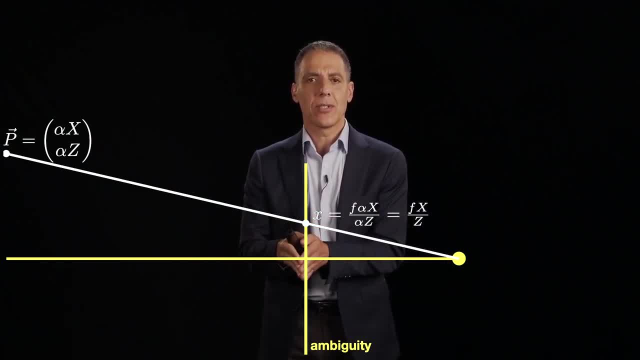 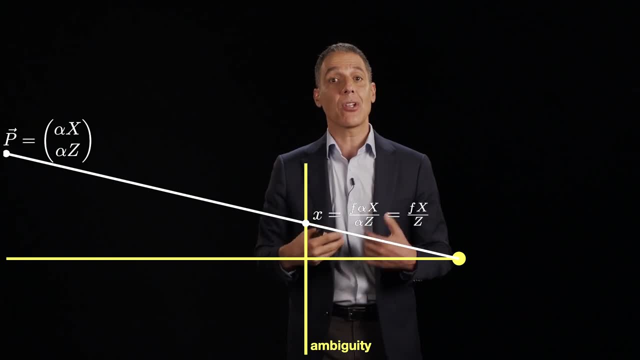 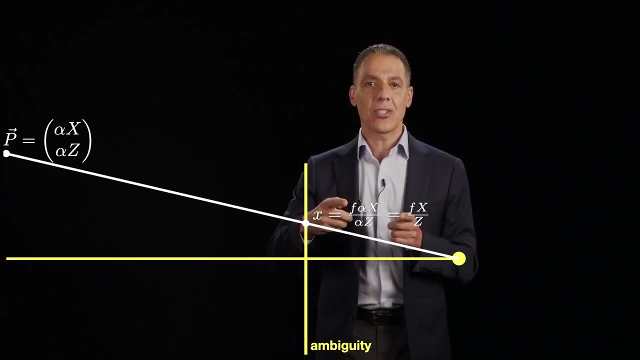 and I'm projecting them into a one-dimensional sensor. Eventually I'll take points in a three-dimensional world and project them into a two-dimensional sensor. There is a loss of information. There is an inherent ambiguity in the size-distance relationship to an image relative to the world. 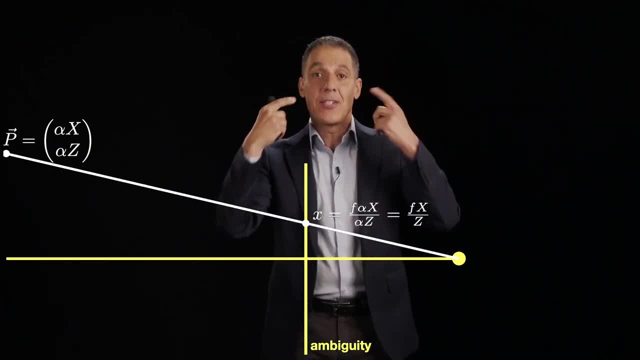 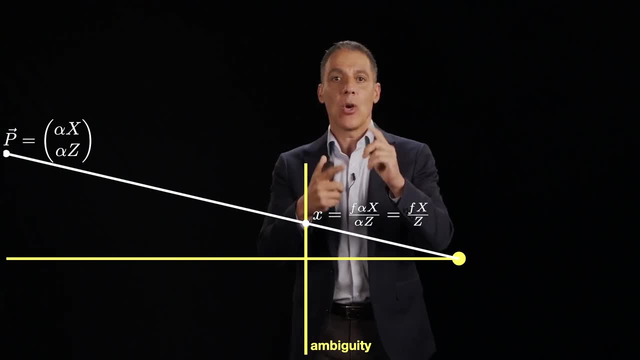 Now the human visual system. this thing right here deals with that ambiguity in a number of different ways. First of all, I have two eyes, so I see the world from slightly different perspectives, which allows me to reason more about the three-dimensional world. 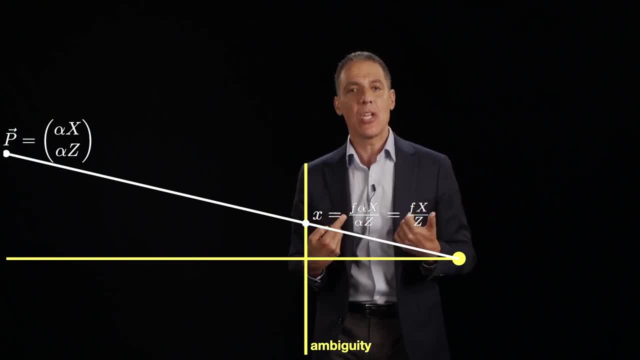 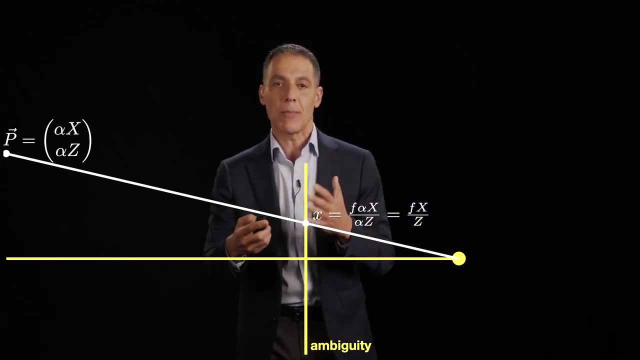 I also have a lot of inherent knowledge about the world. I know roughly how big people are, so I can reason about how far they are. I also can move. As I move, I can reason about where things are in the world relative to my motion.